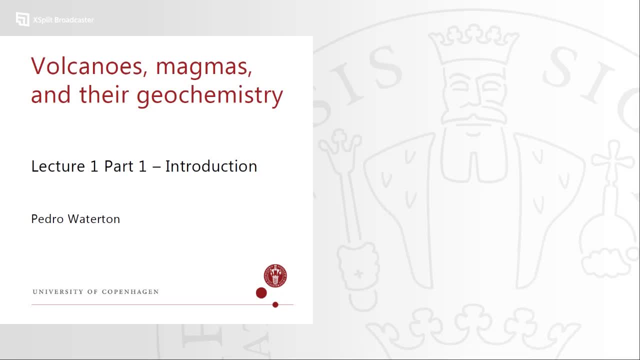 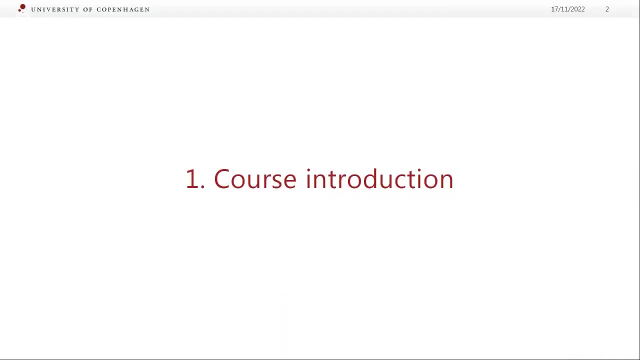 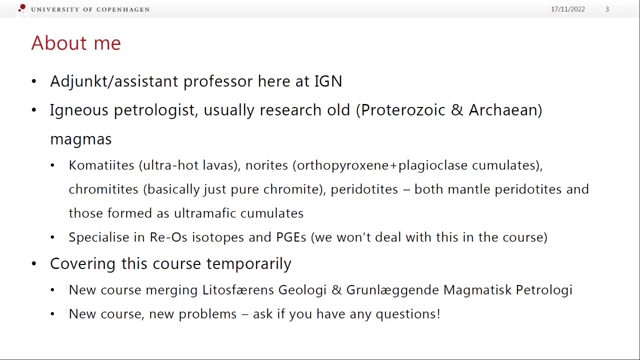 Great Welcome. So yeah, this first lecture is just going to be a bit of instruction. I'll go through some administrative stuff about how the course is going to work And then I'll do a really quick overview of like everything- almost everything- that we're going to talk about. So we'll start with the intro. So just a little bit about me. I'm a precariously employed assistant professor at IGN. I am an 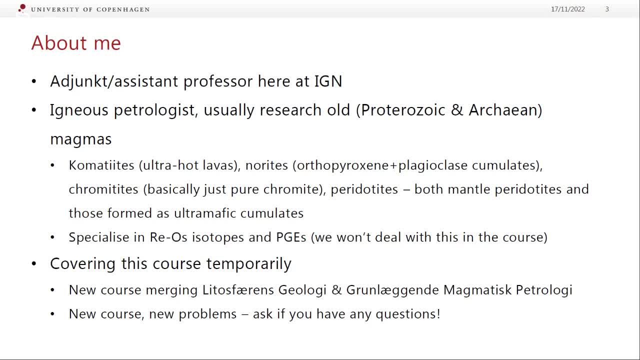 English patrologist first and foremost, also a bit of a geochemist, but I mainly research really really old stuff which unfortunately we're not going to cover too much, which is a shame. It's really cool. So I've done a lot of work on comartii, which are these kind of ultra hot. 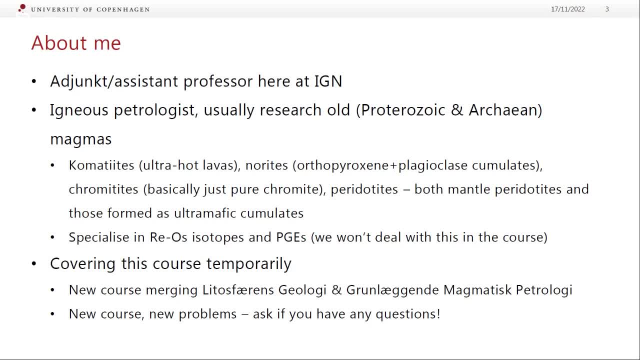 lavas. they don't erupt anymore. The oldest one is 90.. The youngest one's 90 million years old, but the vast majority are older than 2.7 billion years old, And I guess I did my PhD in these fairly special ones from the protozoic. So kind of unusual. 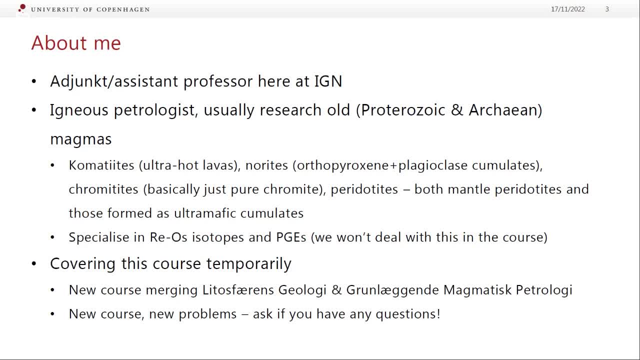 I've also done some work on norites, which are these orthoproxene and plagioclase cumulates that are also. you do see them in the present day, but they're a bit more rare. they're more restricted to an early period of Earth's history. I've worked on chromatites, which are these weird. 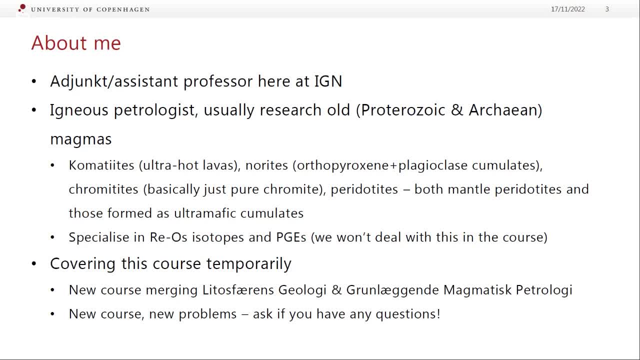 rocks, which is basically pure chromite and peridotites, a mix of mantle peridotites from recent rocks and ultramafic cumulates from the Archean. I'm also a bit of a specialist in reading of isotopes and PGs, and I don't get to talk about them at all in this course, So that's a. 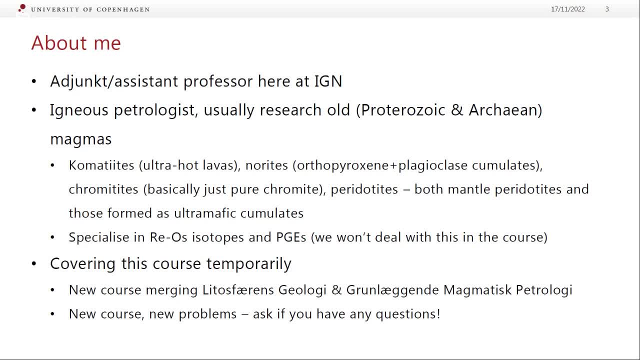 shame. So I've just been drafted in to cover this course for this block. But it is a new course. It's never been done before. This is merging two previous courses, one which was called Grünlegener Magmatis Petrologie, which was more on the kind of magma generation, and 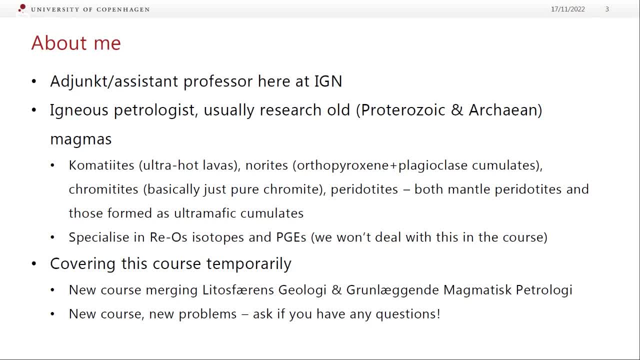 crystallization side of things and another called Littelsferdens Geologie, which was more like tectonic settings a bit more on, say granites and evolved magnets and that sort of thing. So I cannot stress this enough. There's going to be problems. It's a new course I won't have done. 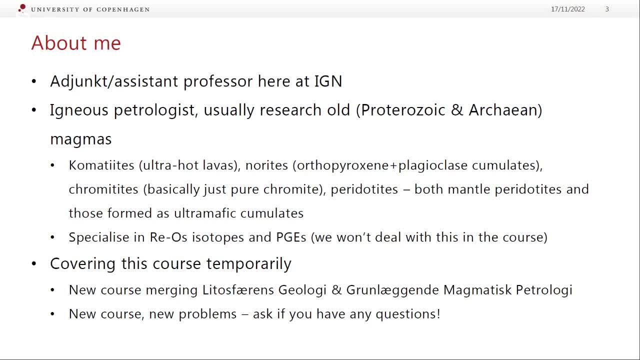 this. I don't know which bits you guys are going to get. well, I don't know which bits you're going to struggle with, So please ask me questions. If you don't understand something, there's a good chance I haven't explained it right or the structure of the course isn't giving you all the basics that. 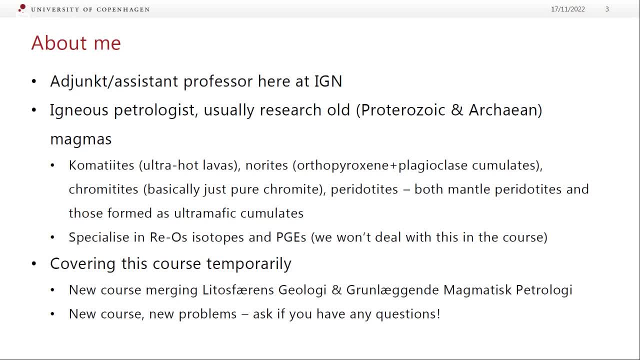 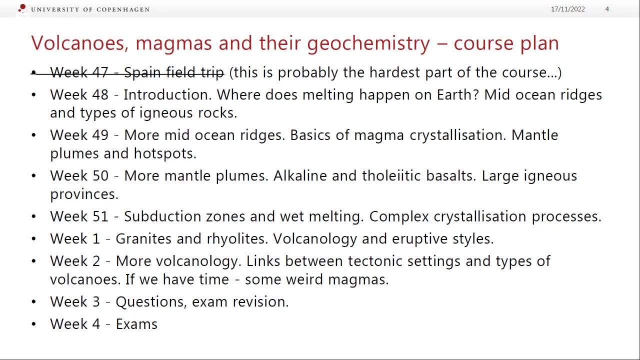 you need to get to understand what I'm talking about, So you have to just be straight up with me. I've got breaks in the lectures where I will stop and specifically ask for questions, but you can ask me any time. Yeah, So don't be scared. All right, The plan for the course. We've already. 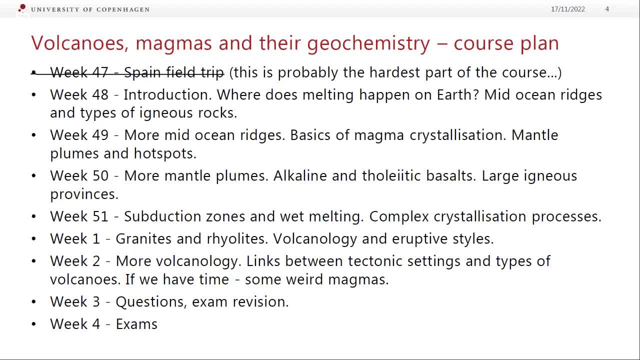 done this Bainfield trip. As I said, it's probably the hardest part of the course And I think the reason for this is you saw a lot of volcanic rocks. A lot of them were very strange. So we had lamprites which are quite weird and complex. We had this concept of metasomatism. We saw some 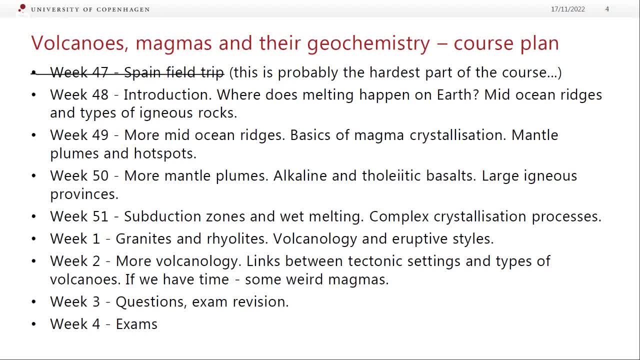 subduction zone andesites, but they were this weird mix of like breccias and columnar jolts, So lots of weird, weird stuff in Spain. So it's all downhill from here. It's going to get easier. So this week I'll do this introduction. I'm going to talk a bit about where melting happens on the 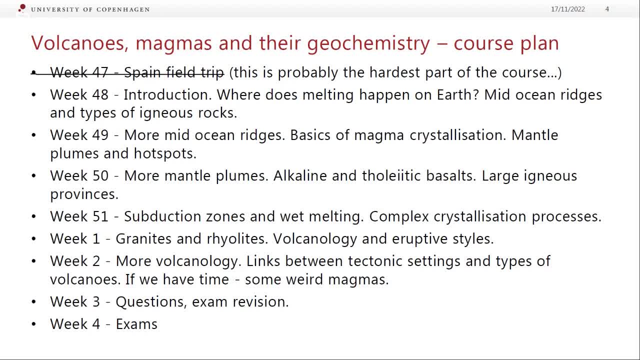 earth, And then I'm going to zoom in on mid-ocean ridges and use those to talk about different types of mafic igneous rocks. After that, next week will be a blend of mid-ocean ridges and some mantle plumes And we're going to use that to talk about. 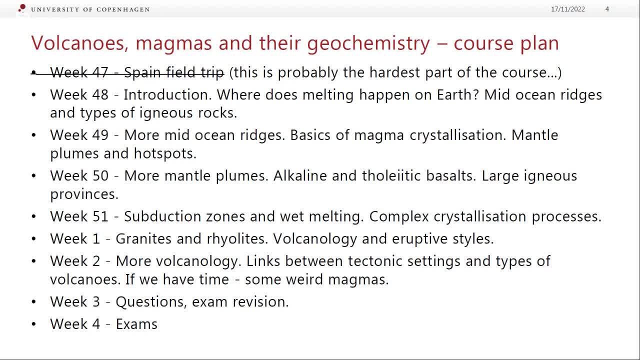 Magma crystallization The following week. after that a bit more mantle plumes, ocean island basalts, comparing alkaline and tholeitic basalts, And we'll talk a bit about large igneous provinces. Then we'll talk about subduction zones and some more complicated. 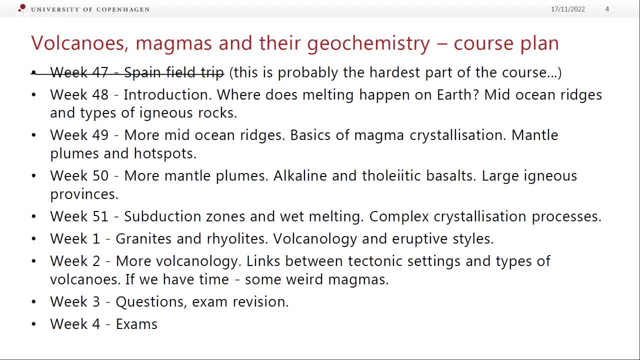 processes that we can have when we're making and crystallizing magma In the new year: granites and rhyolites. So these are kind of more evolved magmas, felsic magmas. We'll talk a bit about that And then finally we'll do a bit more about volcanology and try and bring it all back. 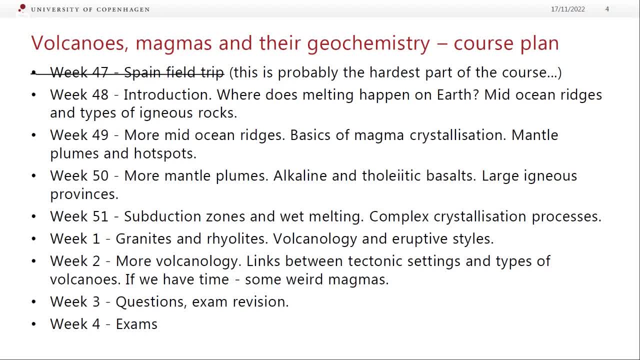 together in the context of the different tectonic settings that we've spoken about. If we have some time, we'll talk about weirder magmas, But that's just nice to have. Yeah, Week three: we'll basically just have a short recap lecture. I'll leave the time for you guys to ask questions In the 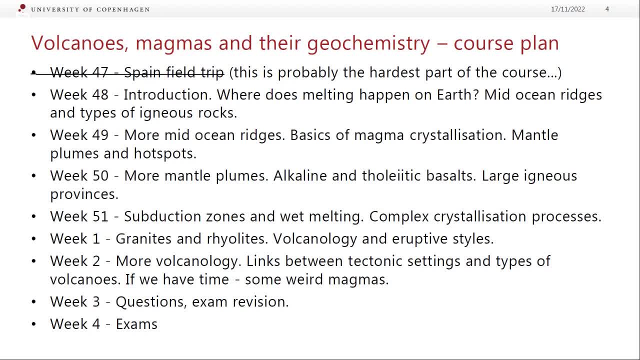 practicals. I'll be there and you can come in and have a look at some of the rocks that we've discussed, And then the exercises, if you don't understand any of the calculations, that sort of thing. So that's just to get you ready for the exam. And then week four is exams. 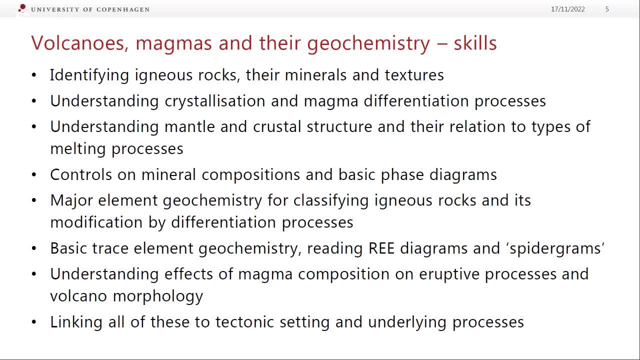 In terms of the skills you're going to learn. I think this is probably non-exhaustive, but these are the main ones. So identifying different types of igneous rocks, the key minerals, the sort of textures you might see. Hopefully we're going to understand crystallization and 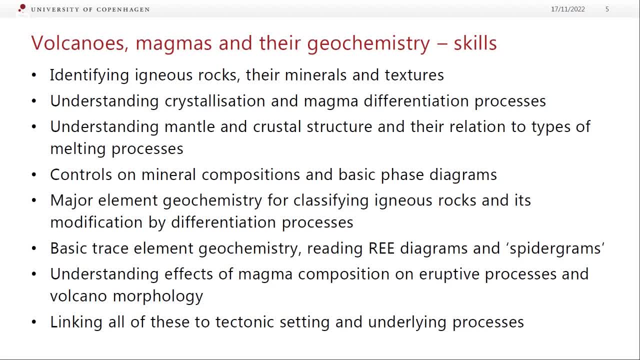 magma, differentiation processes, Mantle and crustal structure and the way this influences melting. We'll talk about mineral compositions. We'll do some basic phase diagrams which I can't remember if you've encountered or not before. So we're going to start right from the bottom. Major element: geochemistry: trace element. 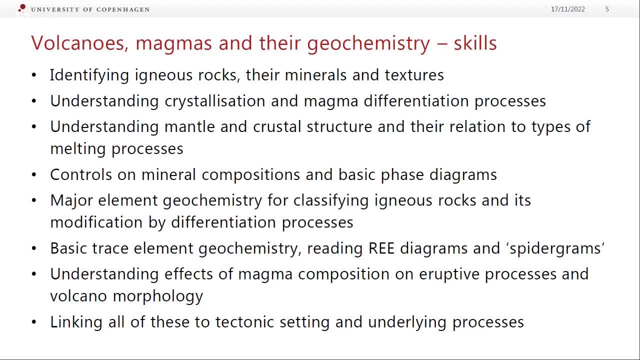 geochemistry, And then we're going to kind of link all these different variations in magma composition and try and understand how that influences volcano types and the way they erupt. Yeah, And then we're going to put all of this in the context of different tectonic processes- Great. 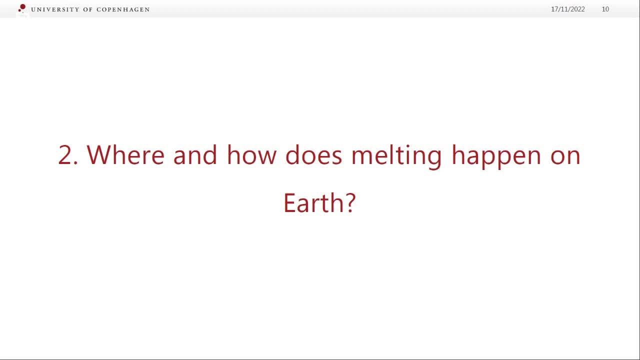 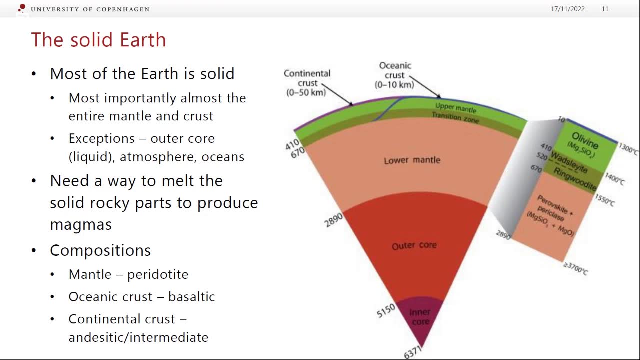 So we'll just do this is like the whole course in one. We're going to do where and how does melting happen on Earth? So hopefully you already know that most of the Earth is solid, pretty overwhelmingly solid And, most importantly to this course, almost the entire mantle and the crust is 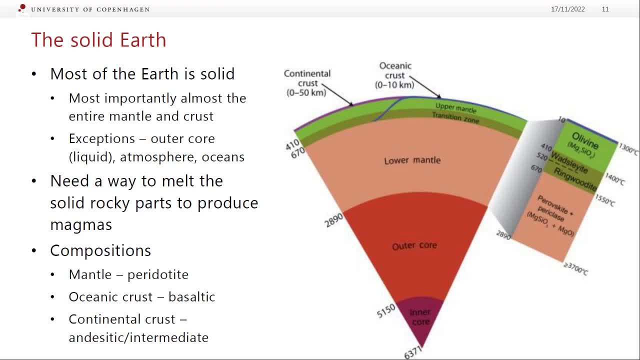 more or less solid. The big exceptions here is: the outer core is completely liquid And obviously the atmosphere is gas. The oceans are liquid, That's fine. So when we talk about making magmas and volcanoes, we need a way to melt the solid rocky parts to produce magma And eventually that's going to erupt as lava. 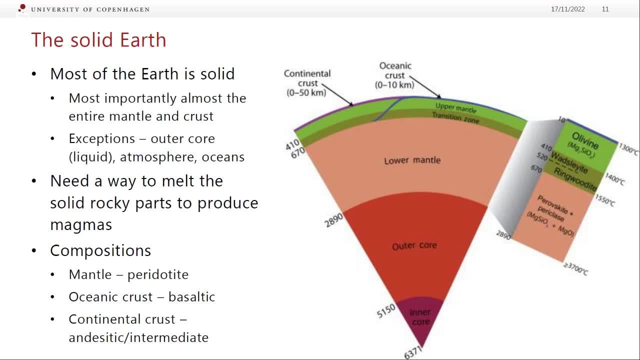 Just in really broad strokes the composition of these kind of different major building blocks. the mantle is made of peridotite. more about that in detail later. the oceanic crust is broadly basaltic and the continental crust is andesitic or intermediate. you might sometimes hear continental crust being referred to as more. 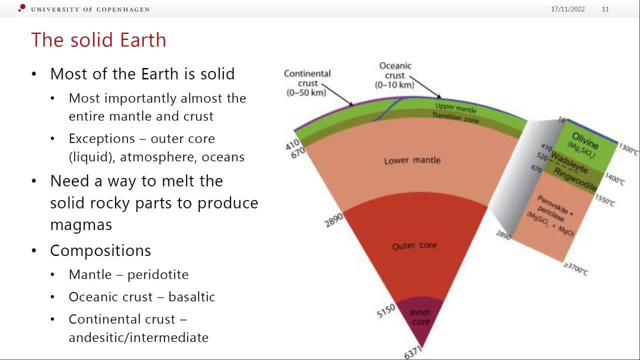 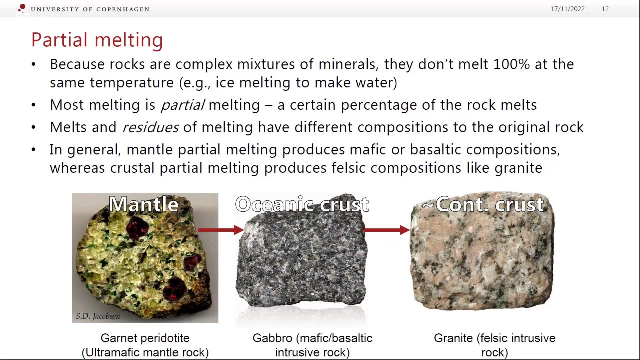 like granitic, but essentially the upper crust is more felsic, a bit more like granite, and the lower crust is actually kind of like quite mafic, so it averages out about intermediate. um so rocks are a complex mixtures of minerals, um so when you melt them, they never. they never just melt all at once. 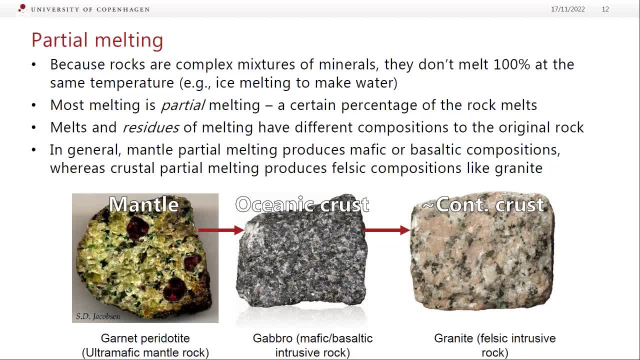 right. if we take an ice cube and we melt it, the temperature- that ice sits there at zero degrees until the whole thing is melted rocks- are completely different. we can start melting at one temperature and we'll get a little bit of melt, and then we could increase the temperature. for 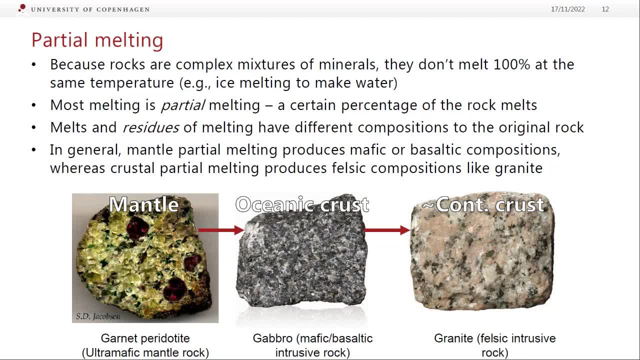 example, it'll melt a bit more and there's actually this, this kind of gap. the? it's completely solid at the top of the ice cube. that's when you first get the first tiny little bit of melt. it's completely molten at the liquidus. um, so most melting on earth is partial melting. it's it's really really rare. 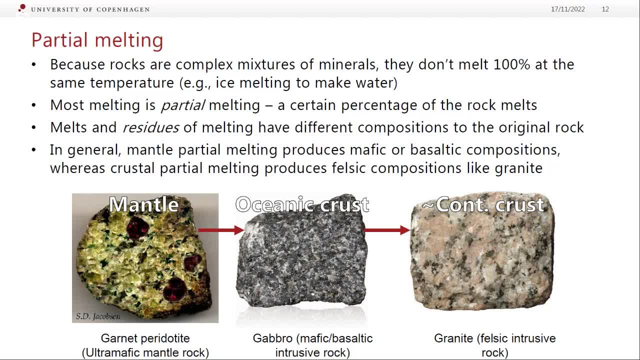 to get 100 melt, and so when we melt a rock, both the melt and the residue that's left behind are different in composition to the original rock. so this is a major way of uh producing differentiation, like changing the composition of things on earth. so in as a really, really rough 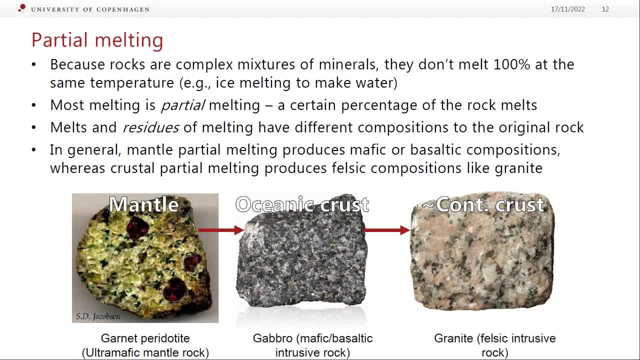 rule of thumb: uh, mantle partial melting produces mafic or basaltic compositions where, as if we melt, the crust will generally produce felsic or more brinetic compositions. um, so you can see, here is that pointing stick still kicking around. where did it go? okay, sweet. 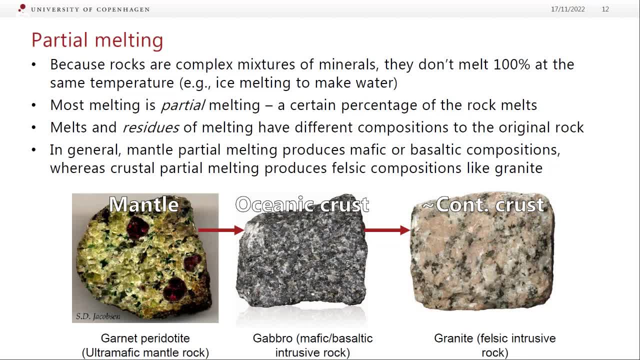 yeah, just really really roughly. this is kind of our progression as we. we start with mantle melt, it makes something more like oceanic crust. uh, here's the gabbro. and if we melt the gabbro then we'll generally get something vaguely granitic and we'll we'll go into way more detail with that later. 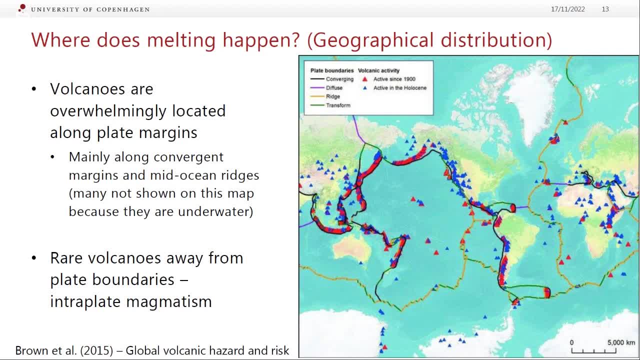 um, so where does melting happen? um, geographically? um, this picture on the right is a picture of volcano distribution on earth. uh, in the resources for this week, i've actually put a poster up there where you can see in like insane detail where the 50 000 odd volcanoes are on earth. 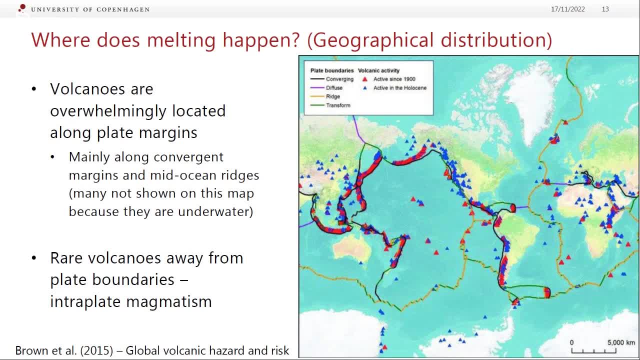 so if we look at them, compared to where plate margins are, they're overwhelmingly along the plate margins, um so mainly along convergent margins. so you can see, um really obviously, the pacific ring of fire. so this is mainly subduction zones around here. there's also a load of volcanoes on mid-ocean. 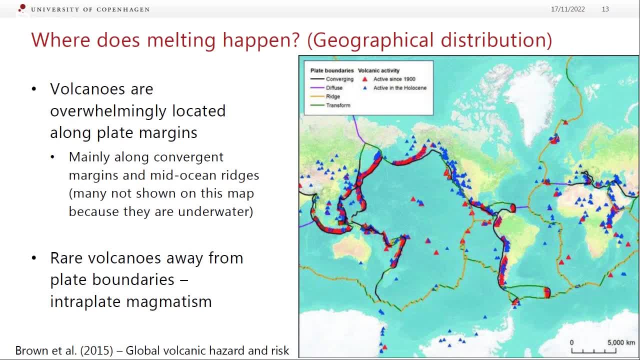 ridges. they're not really shown on this map because they're underwater. um, there are also some rarer volcanoes that are away from the plate boundaries. Good examples: Hawaii over here, some of the other Pacific Ocean Islands and actually a bunch of stuff in the middle of Africa. 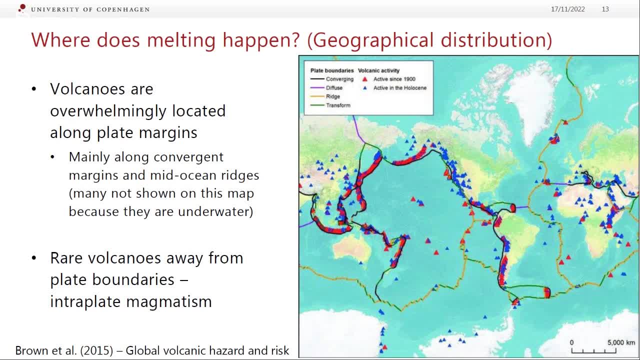 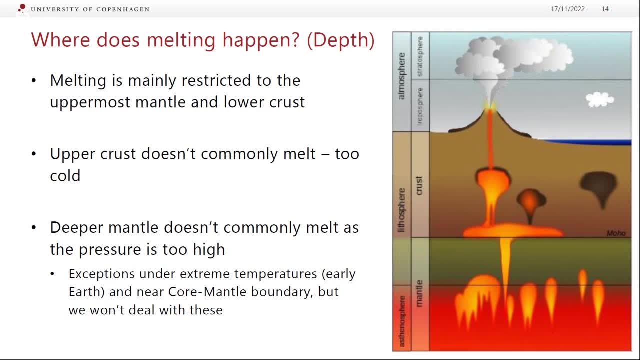 And so this is what we call intraplate magnetism. It's within the plate. In terms of depth, melting is pretty much restricted to the uppermost mantle and the lower crust. The reason for this is in the upper upper crust it's too cold, It's not going to melt. 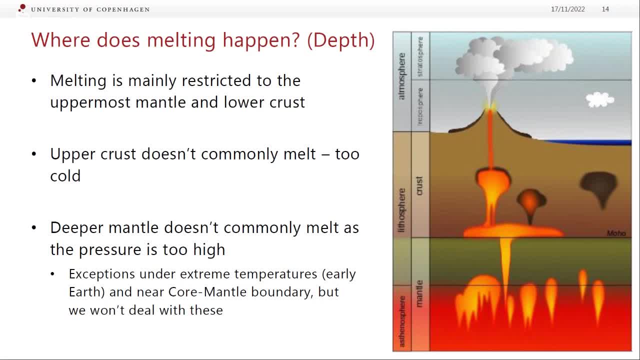 And if you go too deep in the mantle then basically everything's at really high pressure and it's very hard to melt stuff at high pressure. There are some exceptions. So in the early Earth when the mantle was hotter, we might have got melting kind of in the deep mantle. 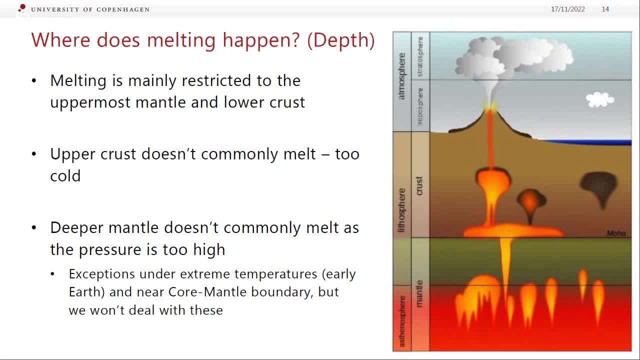 This is a bit controversial And even today, near the core mantle boundary, basically, the core is so hot that it looks like there might be little layers of melt down in the lower mantle. But these are beyond the scope of this course. You don't need to worry about it. 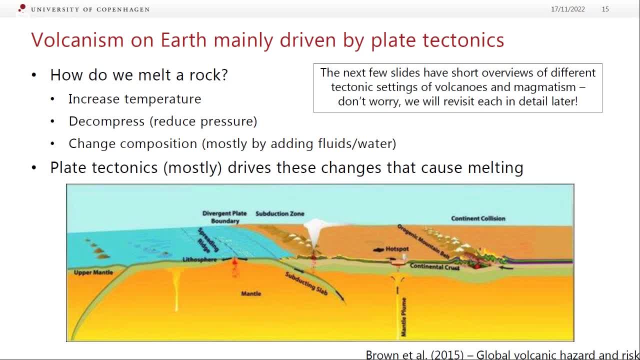 So, thinking about the fact that our volcanoes are concentrated along plate boundaries, we can see that volcanism on Earth is mainly to do with plate tectonics, And there's basically three main ways of melting rocks, and these are mostly driven by plate tectonic processes. 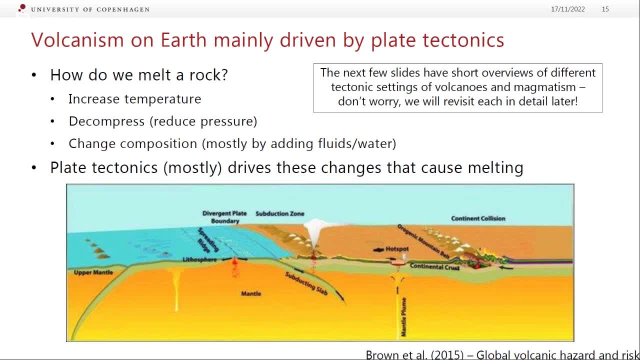 So the most kind of obvious one would be to increase the temperature. This isn't as common as you might think. So the second and third are global. We're going to be more what we're dealing with here. So you can decompress a rock. 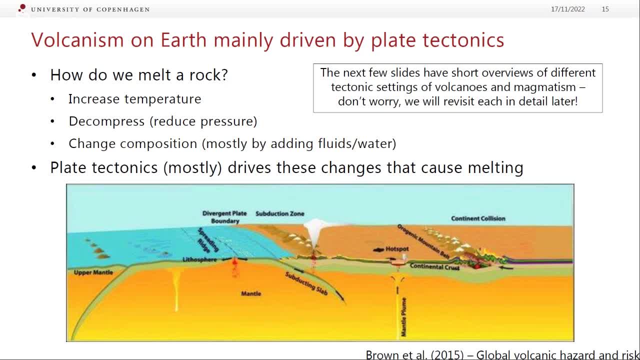 So if it is at high pressure and you reduce the pressure, it will melt, Or you can change the composition such that you make a new composition that has a lower melting temperature. This is mostly just by adding water or fluids. Yeah, I've said it. We're just doing quick overviews of the different tectonic settings. 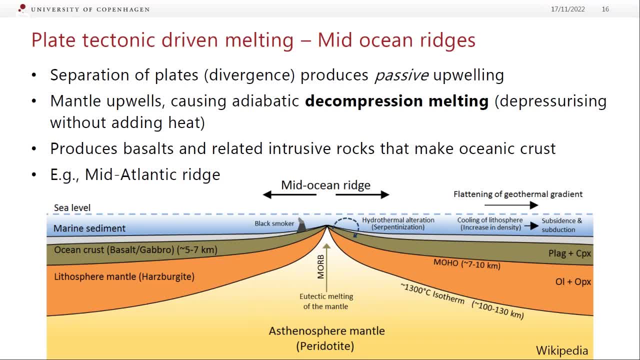 We're going to go into these in way more detail. So a good example of decompression: melting. So this is mid-ocean ridges. So what's happening at a mid-ocean ridge is that the two plates are moving apart or diverging. 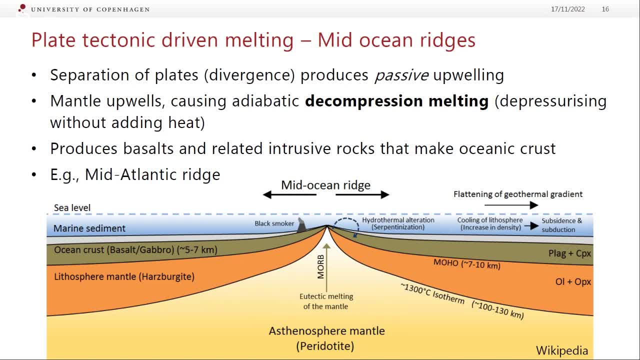 And this produces something called passive upwelling. And what I mean by passive upwelling is there's no force like pushing the mantle upwards. Basically, the ridges are splitting apart. You can't have a gap Right, And so the mantle has to flow up to fill the space that would be left by the plates moving apart. 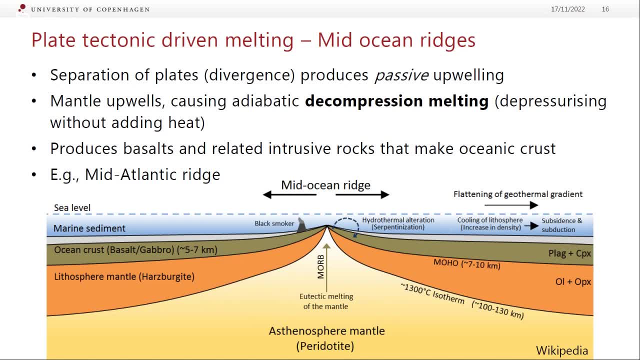 So, more specifically, This is usually called adiabatic decompression melting, and it's adiabatic because we're not adding heat to it. So this is the. It's the same idea as when you go high up in the mountains: it gets colder. 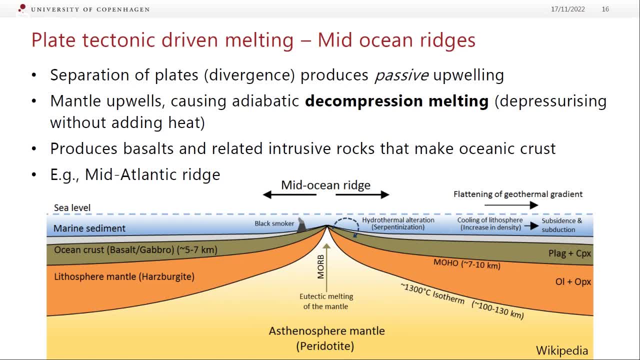 You haven't pulled heat out of that. You just drop the pressure. So this produces basalts and related intrusive rocks that make oceanic crust. There's a ton of examples. Mid-Atlantic Ridge is pretty famous. There's the Southwest Indian Ridge. 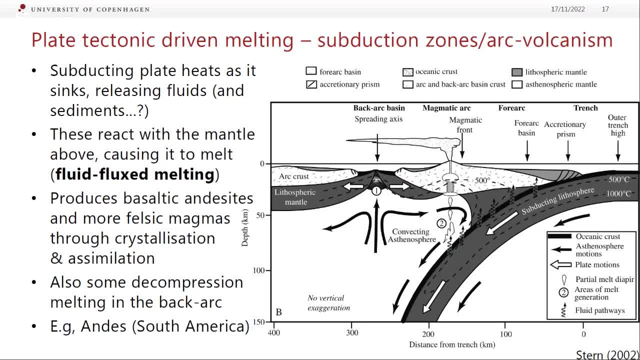 Yeah, they're kind of all over The globe. The next thing we'll talk about is subduction zones. So this is this is a kind of a changing composition, and hopefully you're a bit familiar with this. But what happens is, as the plate that's subducting moves down, it starts to move up. 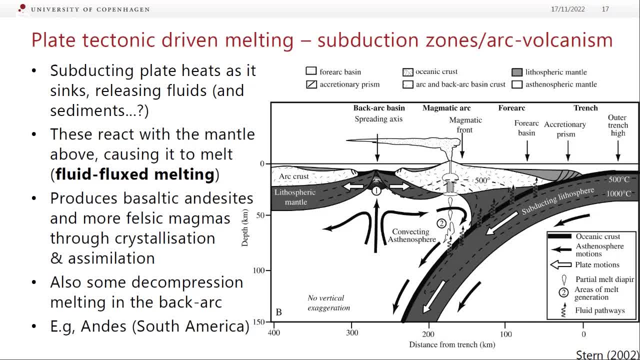 This heat basically breaks down hydrous minerals, release water. the water then reacts with the mantle above. Yeah, I think, yeah, Sorry, there's just minerals that contain water in the structure. Yeah, yeah, Sorry, Is that from the oceans? 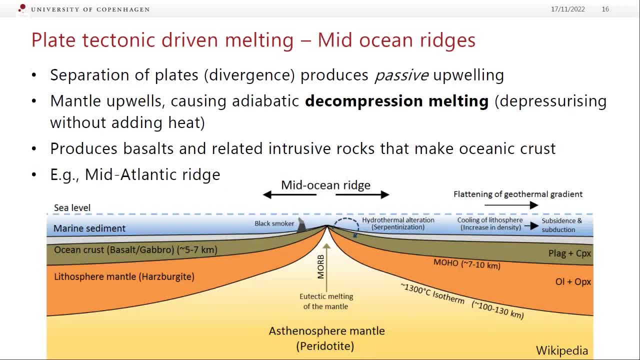 Yeah, yeah. So the the oceanic crust when it's forming a mid-ocean ridge. basically, you're producing all this volcanic rock. they surround it by water. You start generating this really powerful hydrothermal salt. circulation alters a lot of the minerals and creates these hydrous minerals. 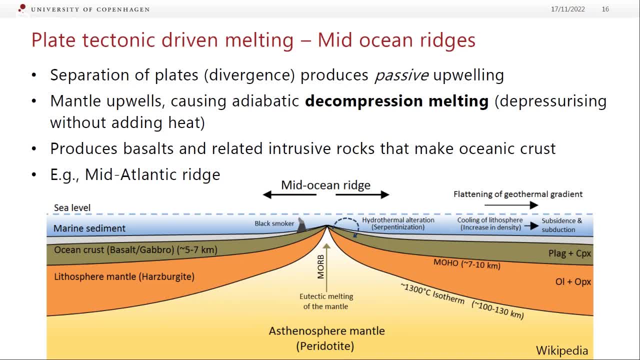 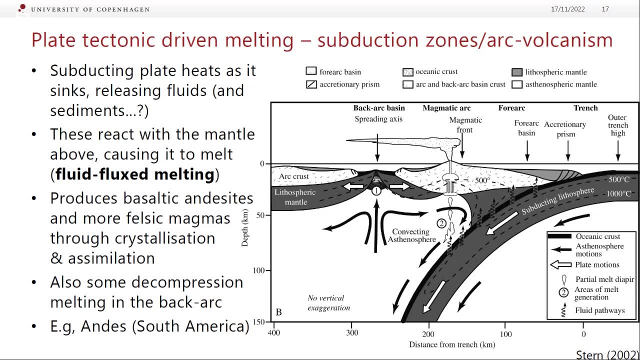 so then, when you subduct those, you basically have a bunch of water stored in minerals that you can release as it heats up. all right, um, so yeah, these fluids react with the mantle, and wet mantle melts at lower temperature than dry mantle, so we call this fluid flux melting it. 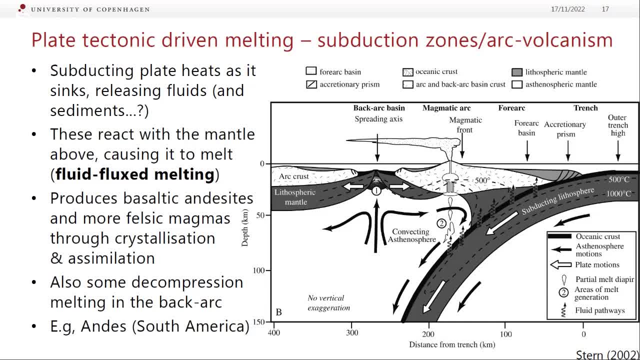 basically, as you're adding water, it's forcing it to melt um at subduction zones. a lot of the primary melts the the first things that we see kind of look like a basaltic andesite or maybe a basalt um. it's a little hard to see because it's subduction zones. we have these really complicated. 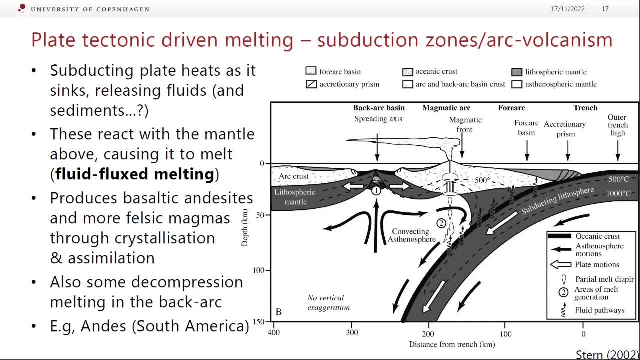 um crystallization and kind of magma plumbing systems that produce a whole range of magmas. the main one is andesite, but we'll we'll talk about more- actually producing more, more felsic, more granitic magmas as well. um, also, you do get a little bit of adiabatic decompression melting in. 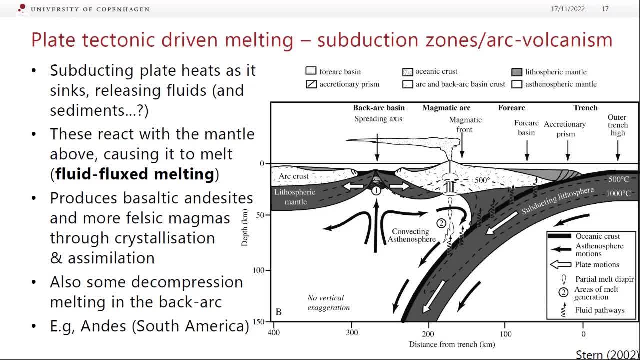 the middle, and then you get a little bit of adiabatic decompression melting in the middle back up. there's sometimes a little bit of fluid in these, but the main process is that you're getting stretching again. so it's a little more similar to the mid-ocean ridge style. uh, best example is the. 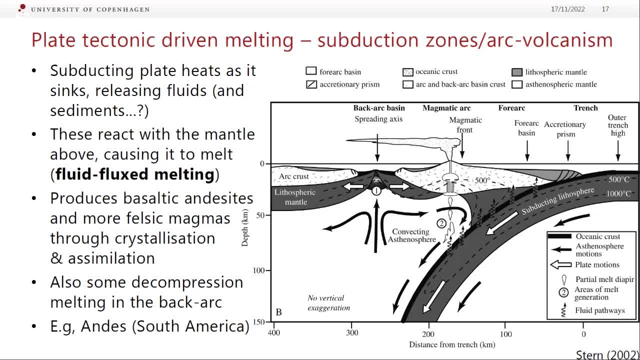 andes, for which andesite is named? uh, because this is just a huge, you know, i can't remember five thousand six thousand kilometers long, uh, arc. yeah, what is assimilation? ah, we will talk about that more later. uh, this is, if you have a hot magma. uh, passing. 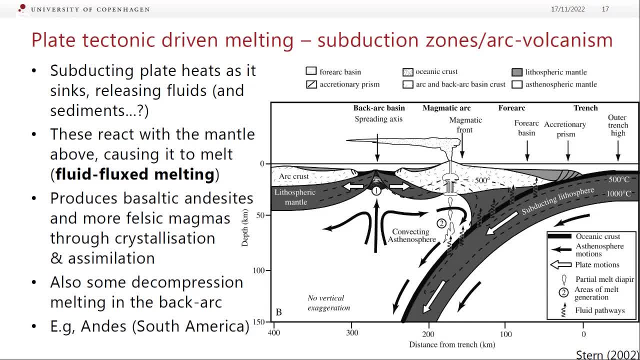 through crust. basically, it can melt it and that melt can get incorporated. so assimilating- uh, you might hear it called contamination as well. um, i tend to use assimilation because contamination has like a negative connotation. this is yeah, anyway, yes, uh, i don't think there's any different. 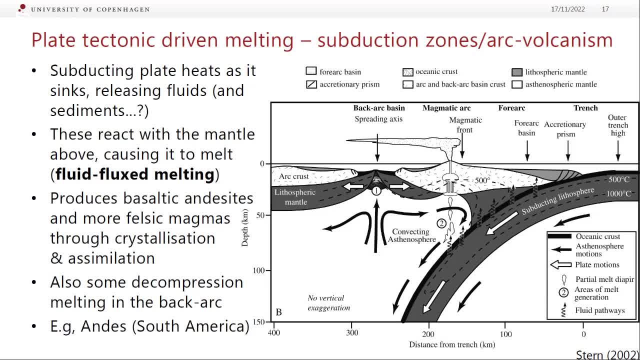 question and then nothing in the background. oh, yeah, so, um. so the second thing comes down and some different questions. yeah, um, the thing that i actually think this diagram has wrong- and a lot of diagrams have wrong, and you probably got taught wrong in first year- is that when the plate's going down, it's not. 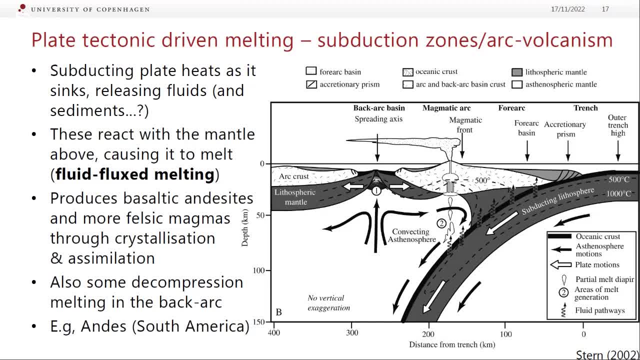 being injected along the angle of the plate, right. so what's actually happening is these things are called they're sinking, so as it sinks the angle, it sinks at an angle that's a little bit steeper than the plate. so if you imagine what that does, over time it actually starts rolling backwards. 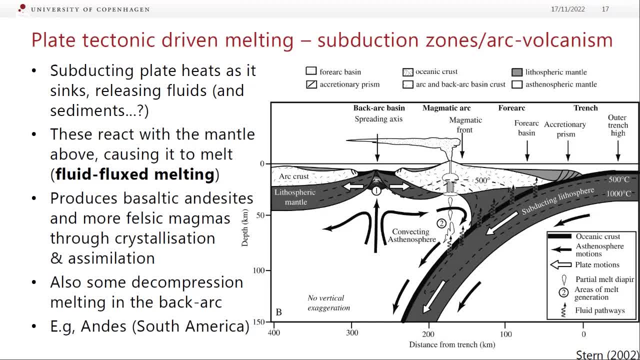 because it's because it's basically falling and so you can't have a gap right. so the arc actually moves out this way and so you're stretching behind it. so most subjections have some sort of backup melting, yeah, yeah, so slab is rolling back and the crust is stretching to accommodate that. yeah, but we'll, we'll, we'll go. 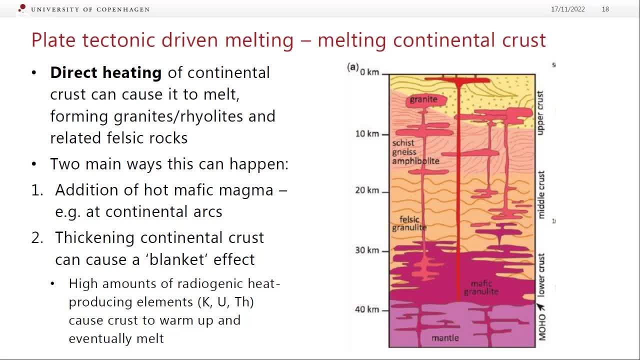 into that in more detail in the in the subduction zone lectures. okay, um, in terms of direct heating, this is, uh, probably the best examples are actually in terms of making evolved felsic rocks in the continental crust. um, two ways we can do that. um, we can add a bunch of hot magma, so this 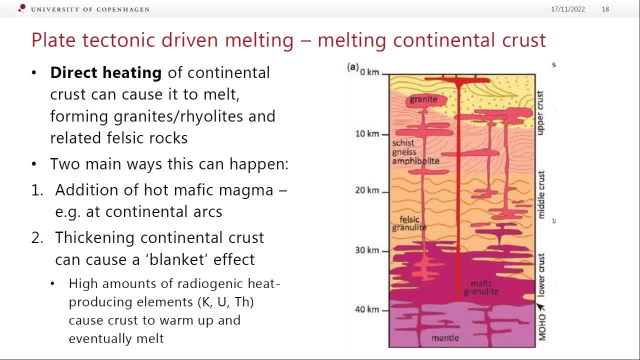 is what happens at continental arcs. we're making a bunch of basalt or basaltic andesite, from this flux melting that's going into the base of the crust and it ends up melting some of the stuff that's there beforehand. so we're adding heat by by sticking a hot magma next to it. um, the other one. 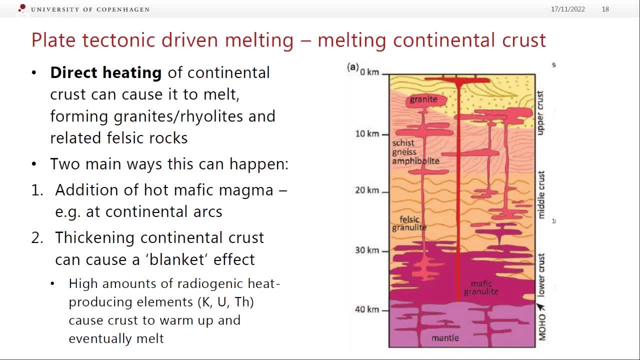 that's, um, yeah, probably is probably most important at collisional zones, places like the himalayas and tibet, is basically, if we, if we thicken continental crust and continental crust is full of these, uh, radioactive elements, then we're basically like building up a really thick electric blanket. 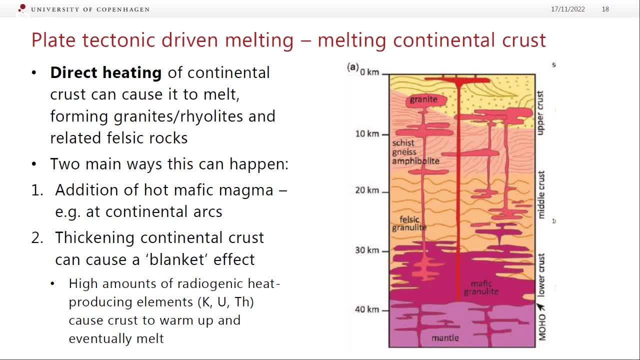 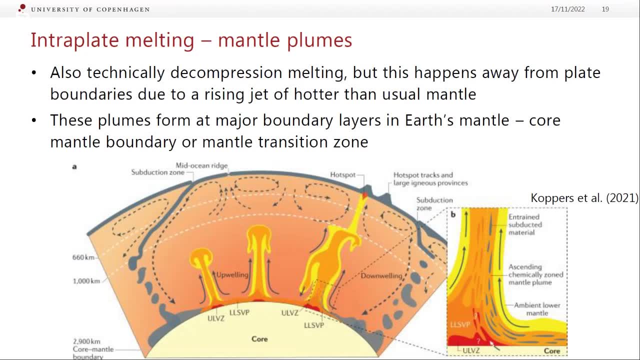 um, where all this radioactivity is heating everything up and it can get hot enough to melt and produce granite. um, yeah, finally, uh, just, there are probably several types of interplate melting, the one we're going to focus on in this course because it's the the simplest and probably one of the more important. 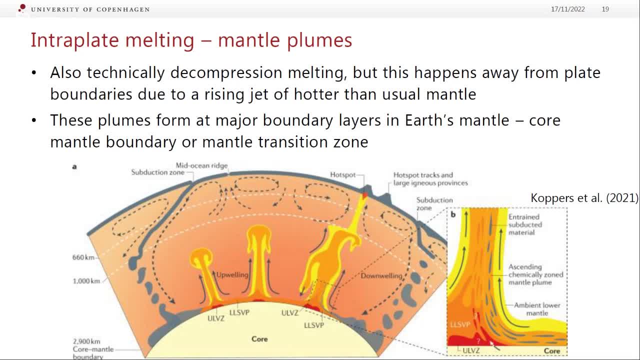 ones, uh, the mantle plumes. um, so where the mantle plume, it's kind of this combination of the- the plume itself is hotter than normal mantle. so plumes are these like hot, uh rising blobs of mantle and so because it's hotter than normal mantle, it will melt more, but the actual melting 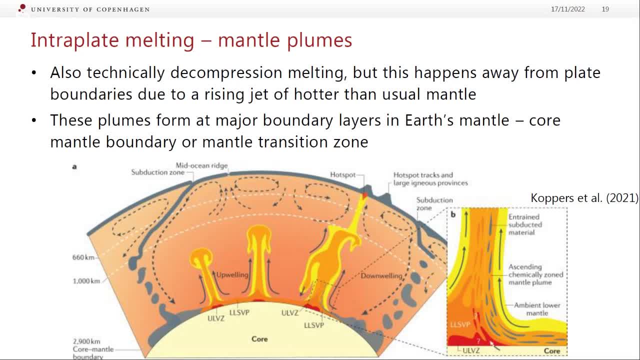 is still this decompression, um, um. so this is, this is still mainly decompression, melting, but you know, hotter than normal mantle. um, the reason we get these plumes is the same reason. uh, if you think back, to say, like high school, if you did convection experiments where you put a 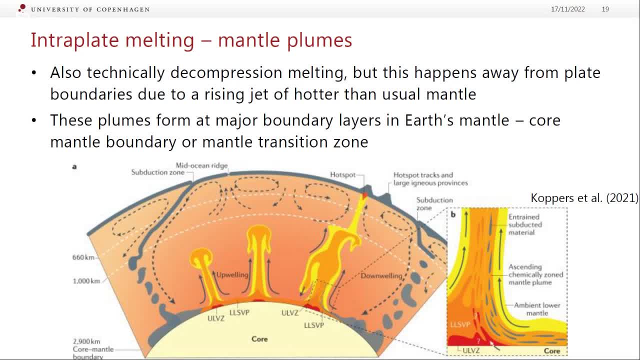 bunsen burner and you add a little bit of dye and you can see it moving around. like that, we're basically heating the mantle from below because the core is really hot, um, and so basically you build up this hot layer next to the core and every so often it breaks off and it 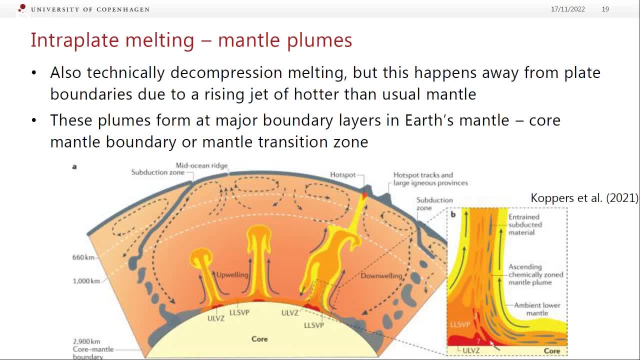 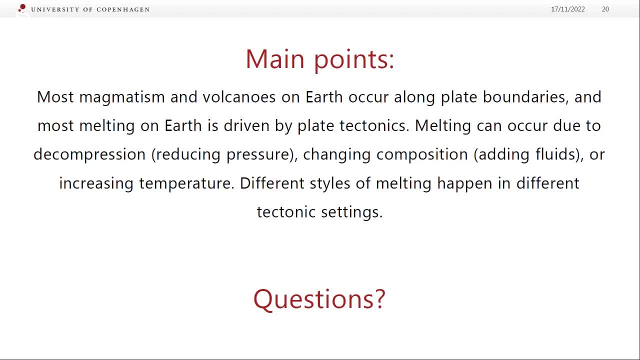 rises up as a jet think like a lava lamp, except everything is solid in this lava lamp. okay, so yeah, just sum up. most magmatism and volcanoes on earth occur along plate boundaries. most melting is driven by plate tectonics, and the main ways we do this is by reducing pressure. 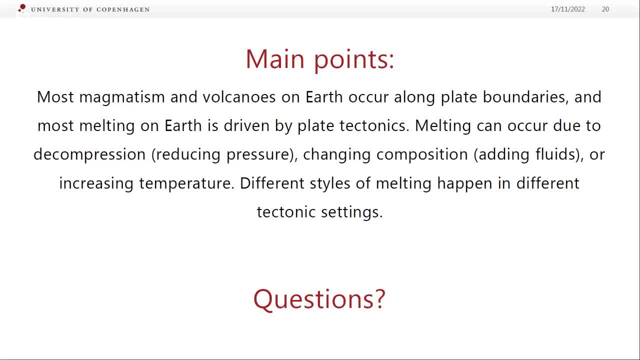 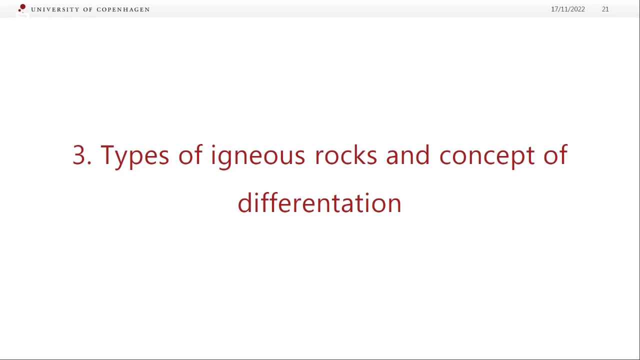 adding fluids, changing the composition or increasing the temperature, and we do see different styles of melting that are kind of associated with different tectonic setting, so i don't have any questions after that. okay, good, so that was, that was the whole course. that's it. yeah, we'll talk really briefly about different types of igneous rocks and 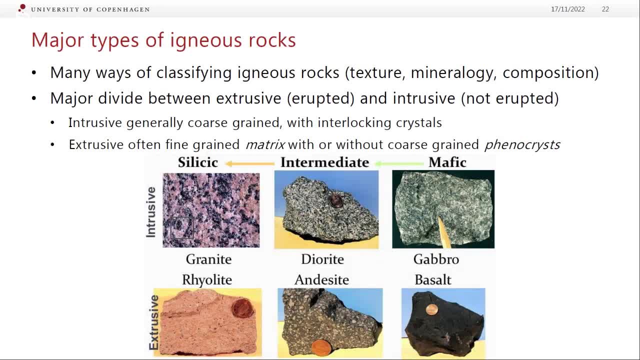 the concept of differentiation that i've already mentioned a couple of times. so loads of different ways of classifying igneous rocks. we can use the texture, we can use the mineralogy, we can use the composition. um, the kind of simplest broad scale divide is that there are extrusive igneous rocks, so these are. 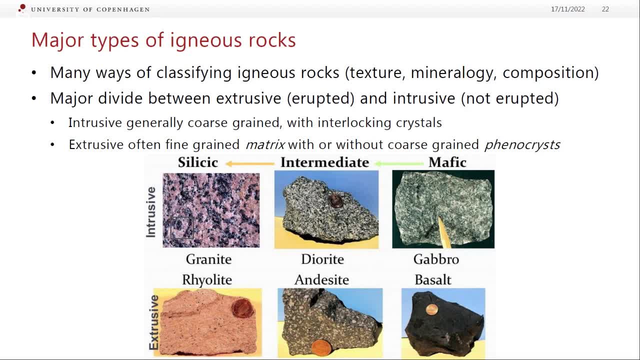 lavas. these are erupted stuff like tufts, ash layers- ignimbrites would fall into that as well- and intrusive igneous rocks that are not erupted. um, if we want to do like a really really broad, like first order distinction, the intrusive ones are going to be coarse grained. 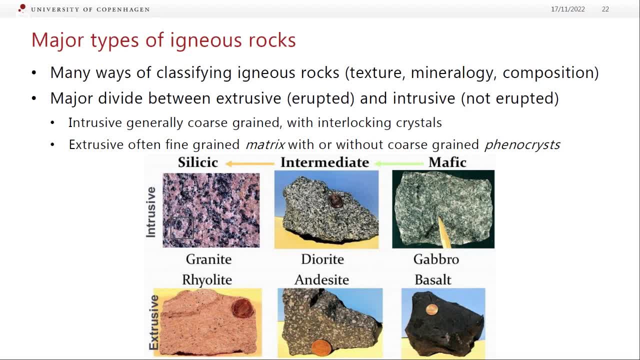 interlocking crystals and that's generally because they've had a longer time to cool. if you cool more slowly, you have time to grow bigger crystals and we shouldn't generally see a fine grain ground mass because the whole thing crystallizes um for extrusive rocks, the typically 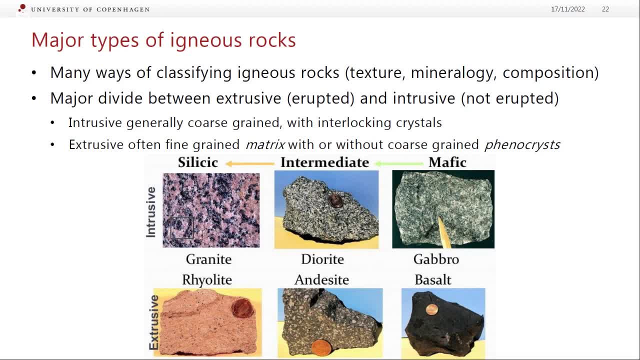 a fine grain matrix. this can be glass, it can be these very, very fine grain crystals and it sometimes they sometimes have coarse-grained phenocrysts, um, so these are like the larger crystals in the fine grain ground mass. yeah, so you can see, on the top we have intrusive and extrusive equivalents, granite's intrusive. 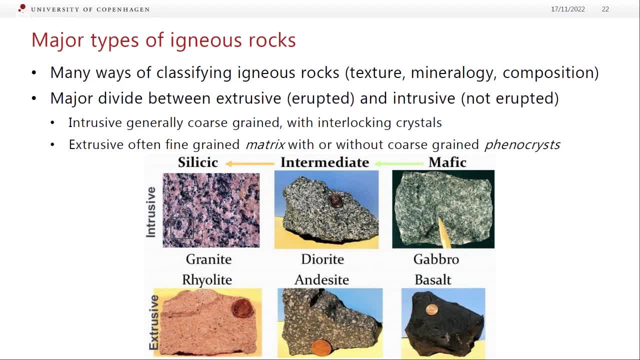 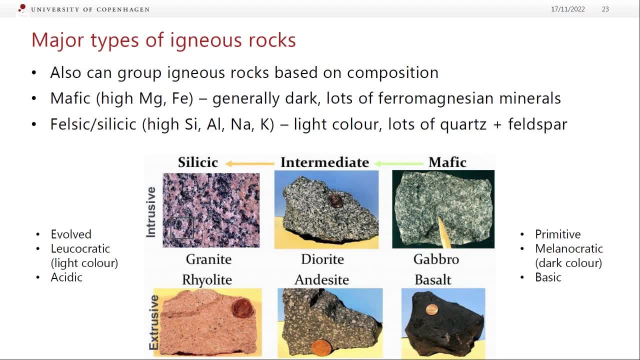 rhyolite's extrusive, uh, diorite intrusive- this is intermediate and the site is extrusive. and then gabbro and basalt, um, we can also classify them more based on composition, which kind of briefly did there. um, generally, when we talk about mafic rocks, these are high magnesium, uh, lots of iron. 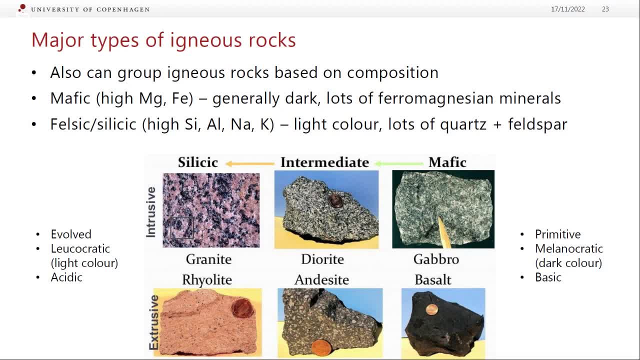 this means that they are often dark because we have lots of ferromagnetic minerals. so ferromagnetic minerals are just anything that has iron and magnesium in it. so olivine would be one, pyroxene would be one. amphiboles are generally ferromagnesian. 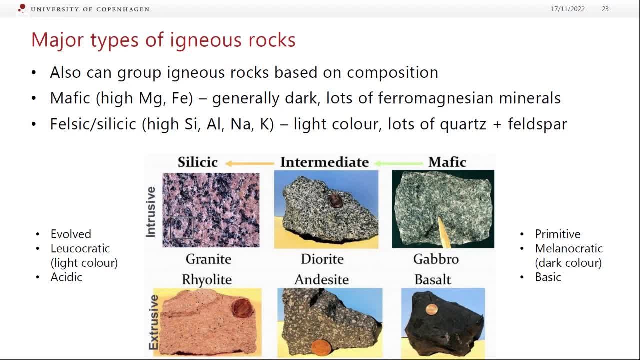 so this tends to give you kind of like a dark colored rock. um felsic or solistic rocks are high in um, silicon, um, aluminium, sodium, potassium, um. and so because we have lots of quartz, lots of feldspars, these tend to be kind of light in color, um. i've put some alternative terms that you might. 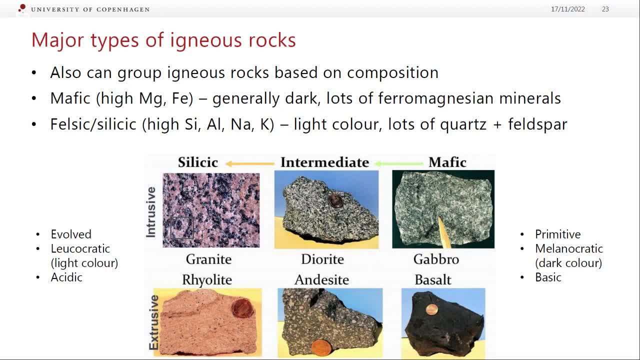 see, um, i will probably interchange a bit between evolved felsic and solistic. i'm really unlikely to call them leucocratic, so i think this is a really dumb word. um, this just means light color, but you might read it in textbooks: um, acidic. this is kind of old school. um, and it's to do with the 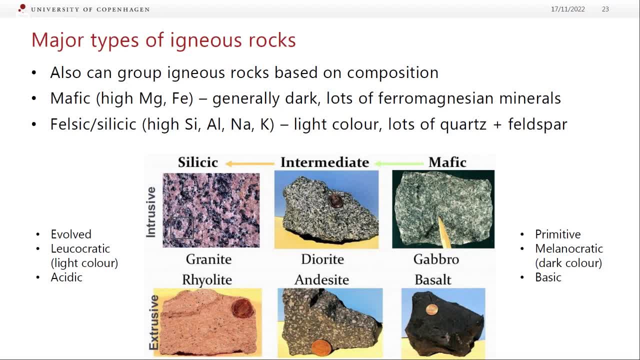 fact that ions like magnesium act as bases. so these rocks are more acidic, these are more basic, but it that's kind of an old school division. people don't tend to call them that so much anymore. on the matrix side of things you might hear primitive. this means fresh from the mantle. 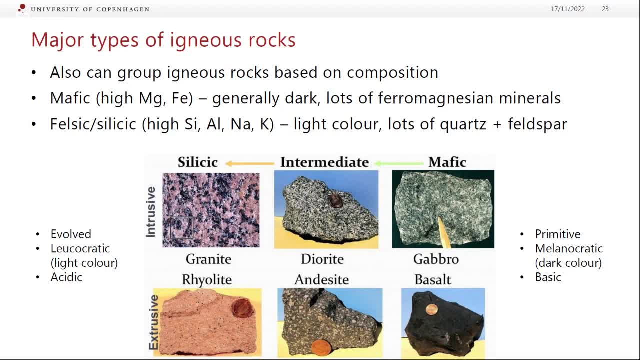 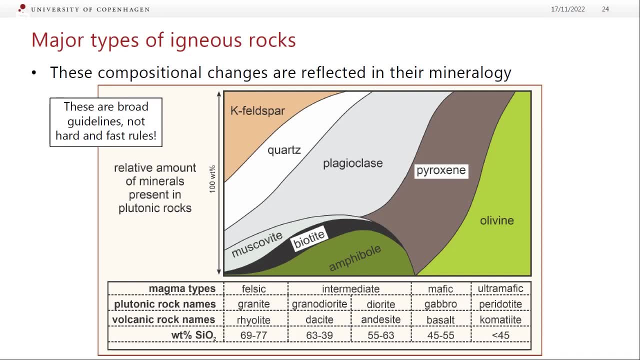 basically i won't use melanocratic. same reason: dumb word, um, basically, um these broad compositional changes, um. this is a really, really rough guideline picture. you shouldn't take this as gospel, but as a rule, in ultramafic rocks we've got loads of olivines. um, in mafic rocks you start to get. 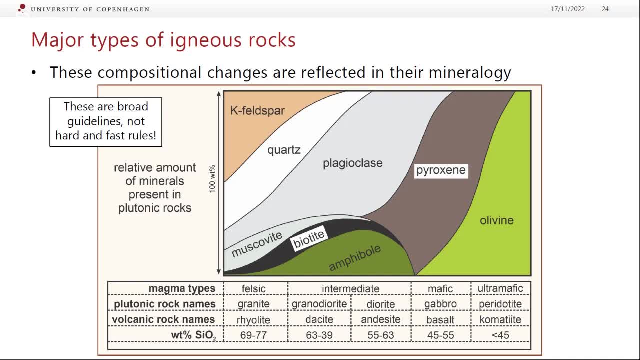 more pyroxene type of place. um depends on the type of rock. sometimes you see pyroxene first. sometimes you'll see pyroxene first, uh, in intermediate rocks you start to get more um and then um. this is kind of your classic granite assemblage of two feldspars quartz and maybe some muscovite. 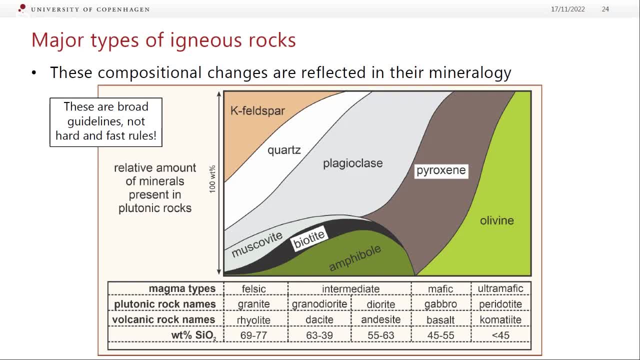 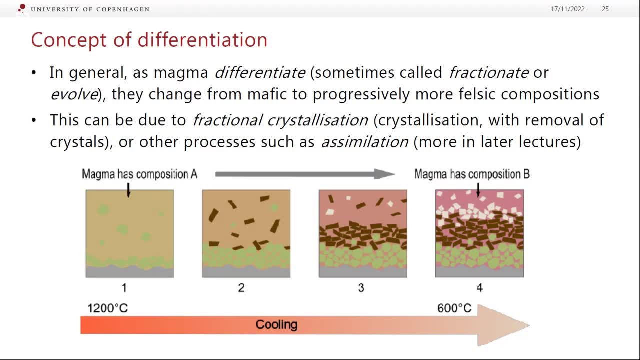 biotype. yeah, so don't take these as gospel. it's really going to vary, so kind of. one of the big concepts that we're going to talk about in this course is is differentiation, um, and so this is the the idea of gradually, uh, processes that change the. 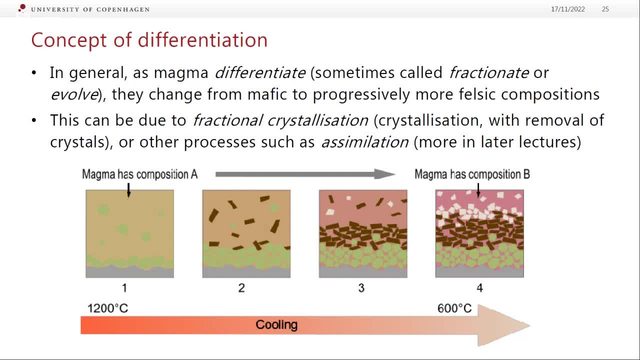 composition, and so this is the the idea of gradually uh processes that change the composition of rocks. so you'll sometimes see this referred to as fractionation or evolving evolution. so, as a magma differentiates, it generally goes from a more mafic composition to more felsic composition. 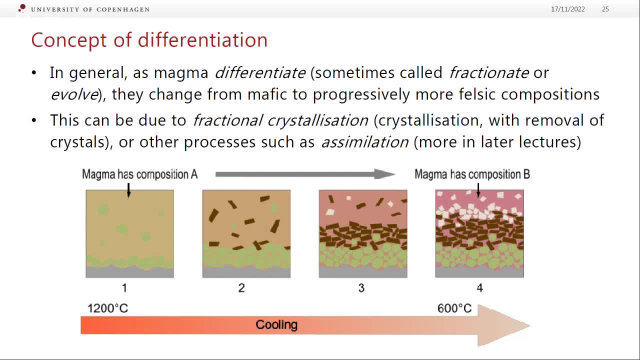 um, this is from a combination of processes. the biggest one is fractional crystallization, which is where it's cooling and crystallizing, and as it crystallizes, the crystals are falling out or being removed from the, from the magma. uh, there's also a combination of processes that are called 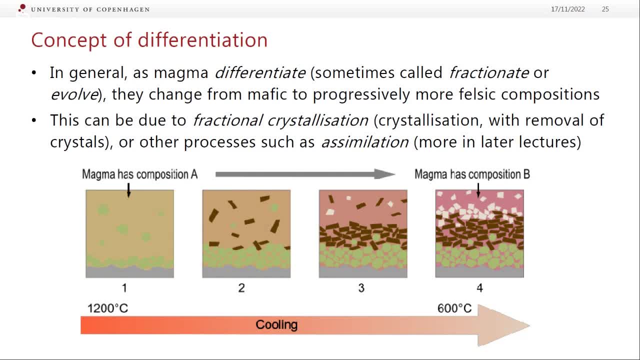 other processes, such as assimilation, which we talked about briefly before. um, so yeah, this is, you know, really schematic thing of we start with basalt, it's got some basaltic composition- uh, i'm going to call these green ones olivine. so it starts crystallizing olivine and these drop out. 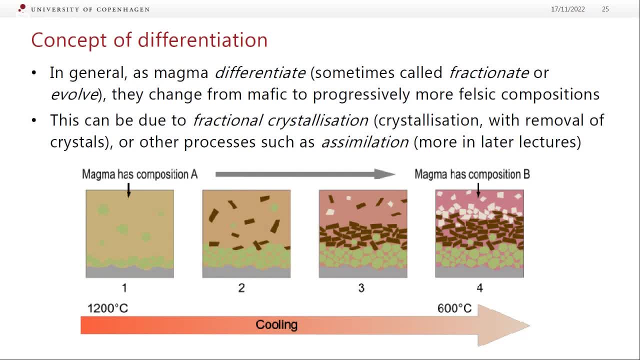 as we remove them, we're removing this olivine composition from the magma. so the composition of the magma is changing and we've got some sort of crystal left behind. um, so maybe it starts crystallizing pyroxene, next algeclades, and over this process as we pull. 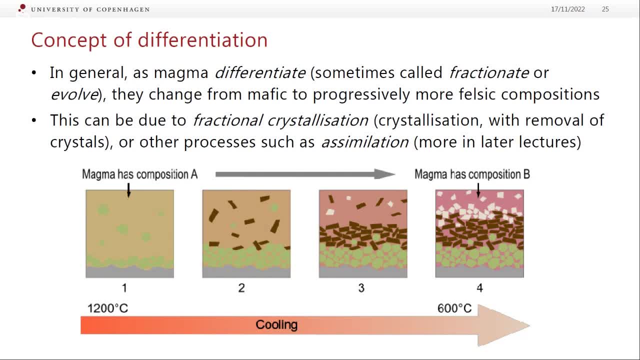 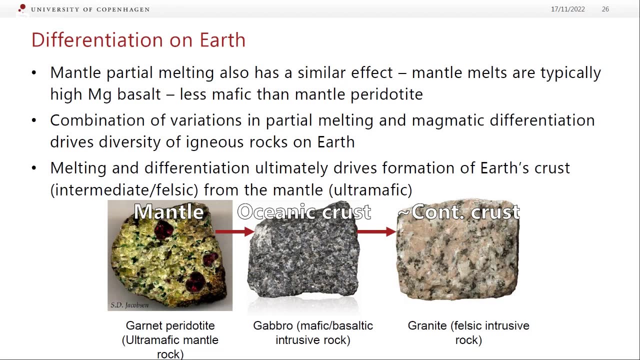 we're left with progressively more evolved or more felsic magmas and some sort of accumulate rocks, uh intrusive rocks that are left behind. so, uh, differentiation on earth is mainly driven by partial melting and uh then fractional crystallization and and assimilation and other processes after you form the magma.